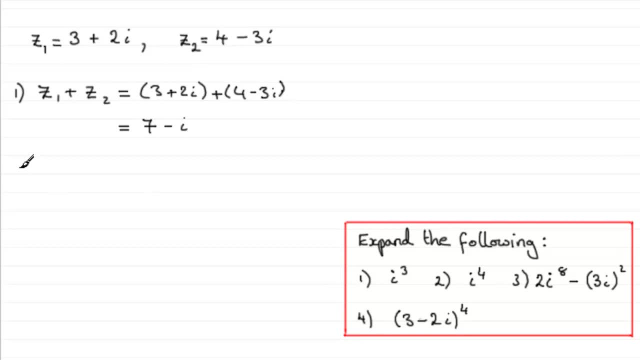 and if it came to subtracting them? let's put this as the second example: z1 minus z2. what would we have now? well, again, it's just going to be three plus two i minus, so then 4 minus 3i. so we end up with 3 minus the 4, which is minus 1, and then 2i minus minus the 3i. 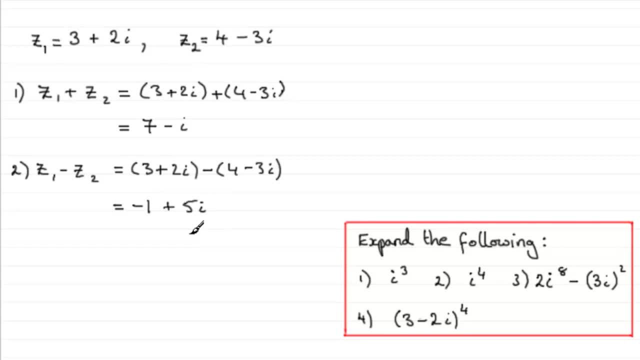 becomes plus 5i, and we don't tend to write the positive term first, the we don't. we don't tend to write this as 5i minus 1. we always write the real part first, whether it's positive or negative, so it's not a good idea to turn this around. okay, so just leave it like that. 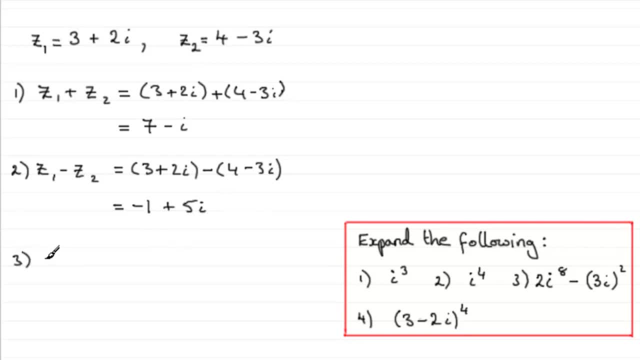 in example three, you can multiply a complex number by another number, a scalar quantity, like, for instance, 5 times z1. 5 times z1, then, would just be 5 multiplied by 3 plus 2i, and what you do is you just do 5 times the real value that's going to. 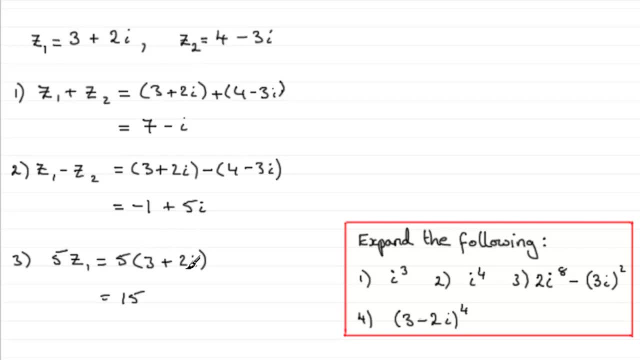 be 15 and 5 times the imaginary value, so it's going to be plus 10i, 15 plus 10i. then, And in part 4, here you're going to find that you're going to come across things like i squared. 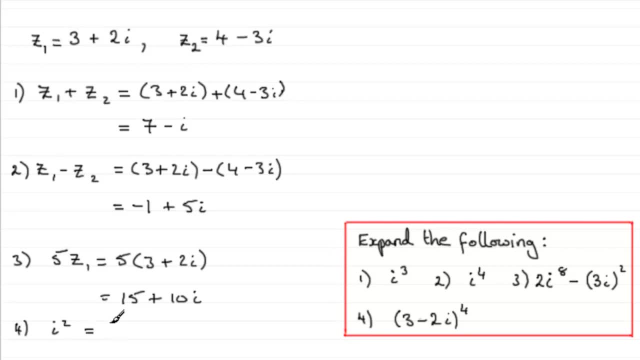 I squared. what's that going to be? Well, we know that i is the square root of minus 1, so we've got the square root of minus 1 multiplied by the square root of minus 1.. And this is going to give us simply minus 1.. Alright, And we'll find that we'll be using this then. 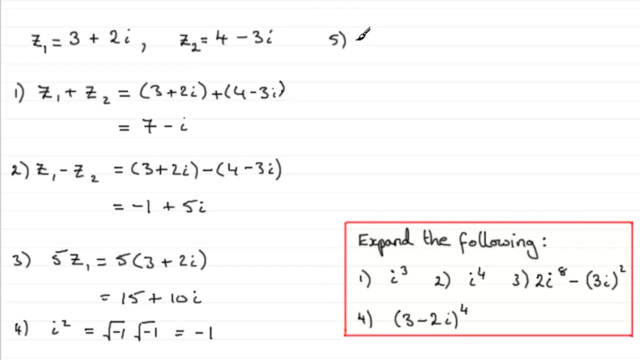 in questions like this. For number 5, suppose we had to multiply z1 with z2.. Then we've got 3 plus 2i Being multiplied by 4 minus 3i, And to do this we multiply out the brackets in the normal. 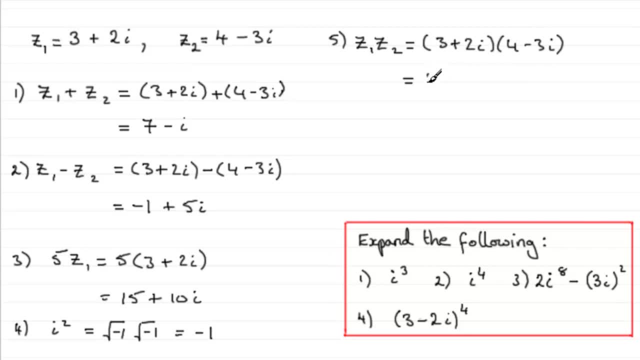 way We start with the 3.. 3 times the 4 is 12.. And then you've got 3 times minus 3i, which is minus 9i, And then plus 2i times the 4 is plus 8i, And then here we've got plus 2i. 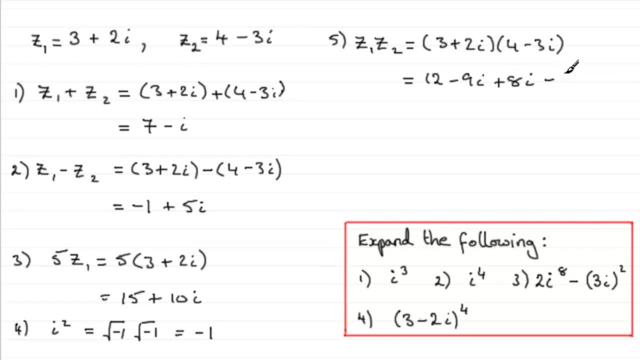 times minus 3i. So that's going to be minus 6i squared. Now we can group together the minus 9i and the plus 8i. That's going to be minus i. So we've got 12 minus i, And then we've got minus 6 times i squared. But 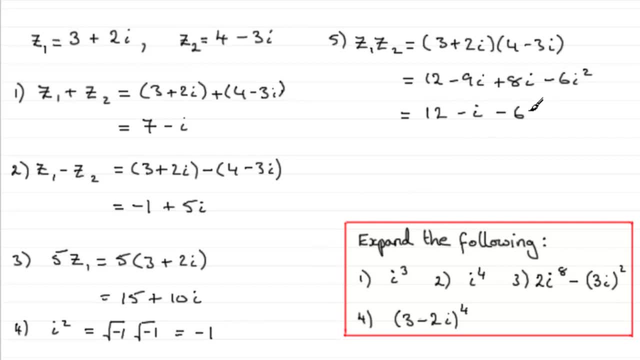 what is i squared? Well, i squared we just worked out down here is minus 1.. So we've got 12 plus the 6 here, which clearly is going to be 18.. And then minus the i, So 18 minus i. Ok. Well, hopefully that's given you an idea, then, how we can add or subtract, multiply. 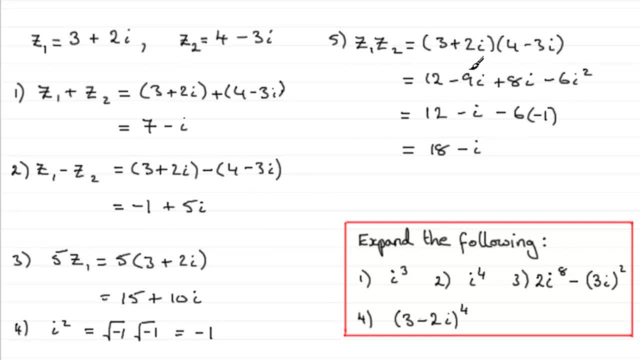 by a scaler and multiply two complex numbers together. Now I've got this short exercise here that you might like to try. You've got to work out what i cubed is. You've got to get the very sort of unit numbers down here as well. 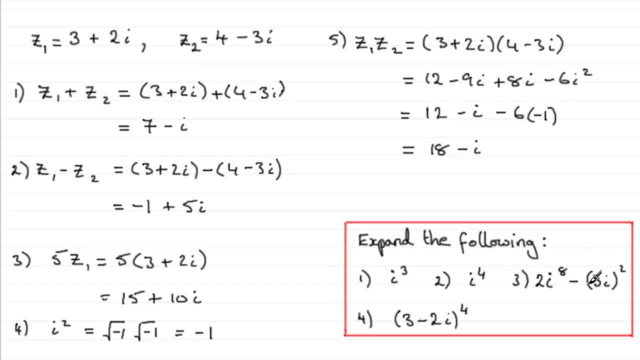 Like this. So you need a logarithmic calculator to do that. You move this over here twice: i to the power 4, 2i to the power 8 minus 3i, all squared, And then in this number, 4,. 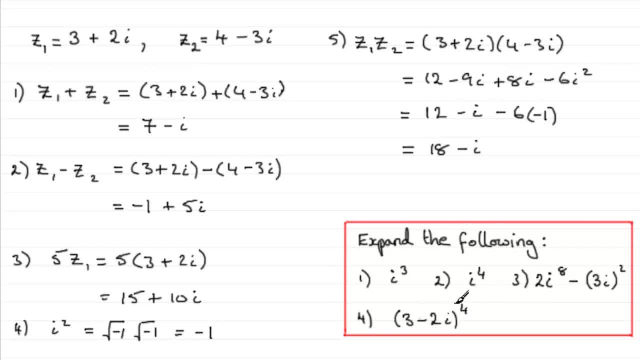 you've got 3 minus 2i, all to the power 4.. And with this 4, you can either do it the long way, which is to write out the four brackets and expand them, or as you'll see me do in. 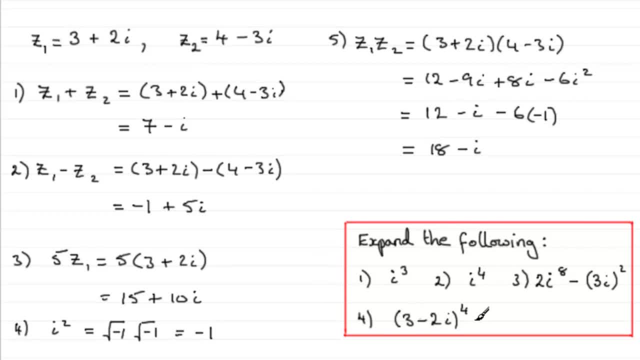 the work solutions. use the binomial expansion. It's a lot quicker. I would definitely encourage you, though, to have a go at number 4, all right, because it brings together a lot of these ideas here. Okay, well, you might like to pause the video. have a go at these and come. 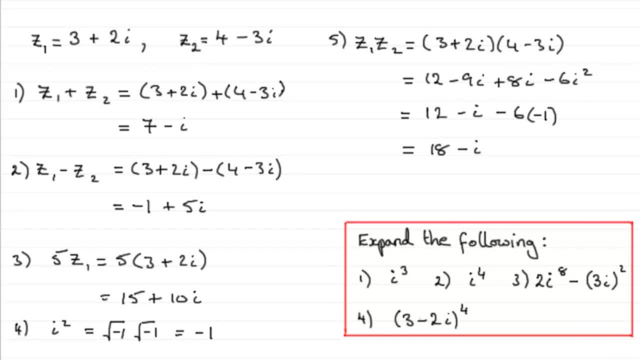 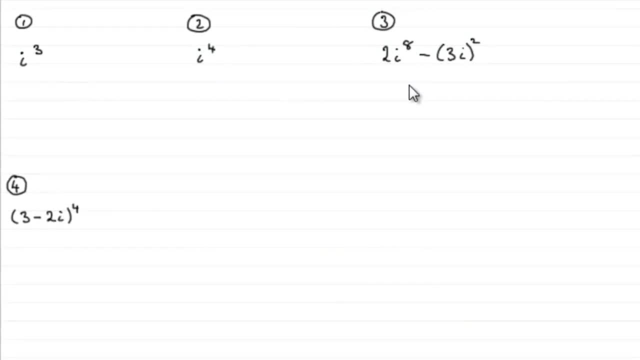 back when ready and we'll run through the work solutions. So welcome back if you had a go at these. Let's see how you got on Well. first of all, then, i cubed. how are you going to do that? 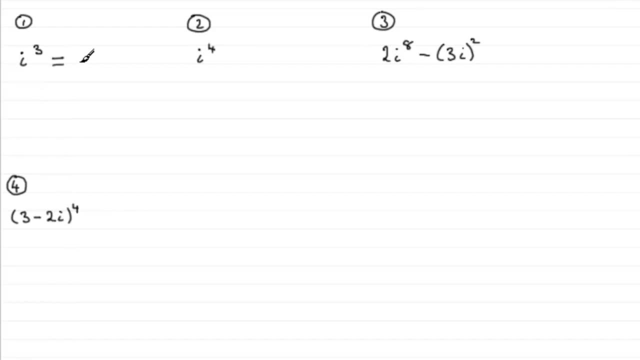 i cubed. how are you going to do that? Well, what you'd need to do is think of this then: as say, i multiplied by i squared, And we know that i squared is minus 1, the root of minus 1 times the root of minus 1, that's. 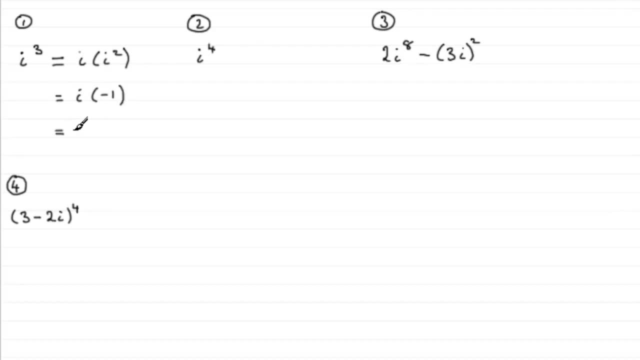 minus 1.. So we end up with minus i, And when it comes to number 2, i to the power 4, well, we can think of this: say: as i squared, all squared, i squared, we know, then it is minus 1.. And so we've got minus 1, all squared. 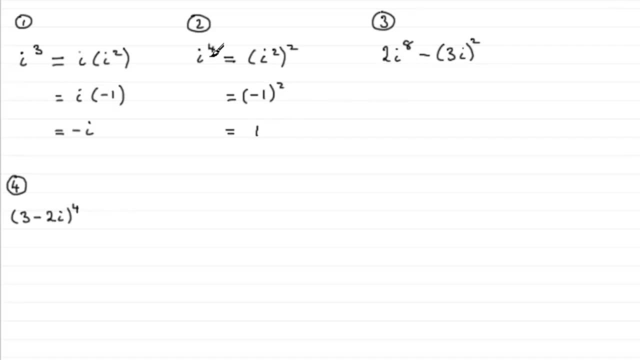 which is clearly going to be 1.. You could do, I suppose, i cubed times i. i cubed, we've seen, is minus i, And if you times that with another i, you're going to get minus minus 1, which is going to be 1, right. 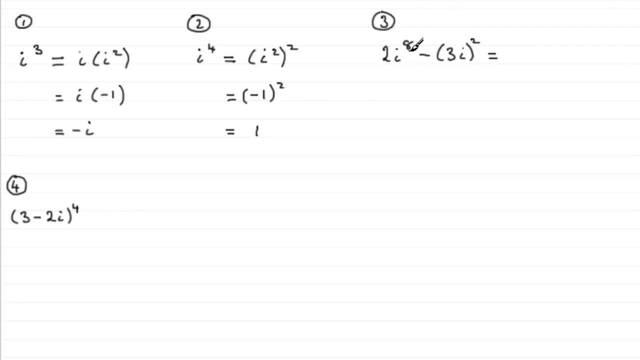 Minus for 3.. 2i to the power 8 minus 3i all squared. well, we've got the 2 and i to the power 8, I would see, as say, i to the power 4, all squared, And then we've got minus 3i. 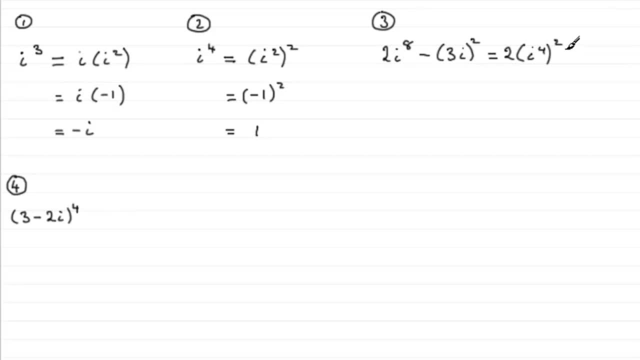 all squared. Well, if we square the 3,, we've got the 9, and then that's going to be multiplied by i squared. So we dozę i squared. that's going to be multiplied by I squared. so we've got. 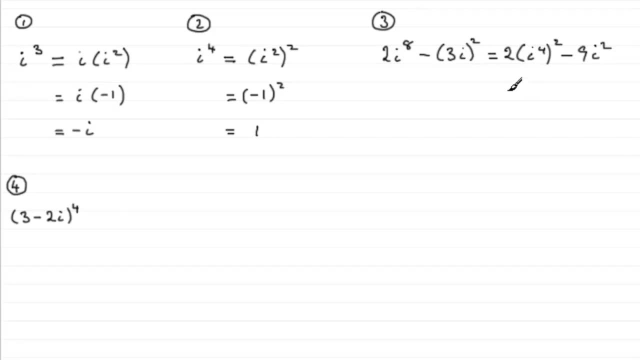 9. I squared there. What is I to the power 4?? We've just seen that it's 1, so we've got 2 times 1 squared. in other words, just simply 2, and for this we've got the minus 9. 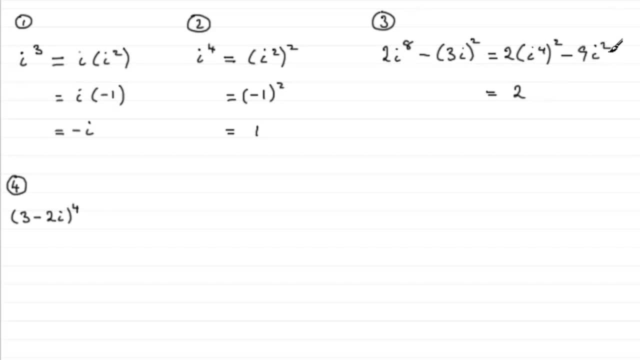 being multiplied by I squared. I squared is simply minus 1. so minus 9 times minus 1 is plus 9, and that's going to give us 11.. Now number 4, this is the one I was particularly interested in because it's going to bring together a lot of ideas. 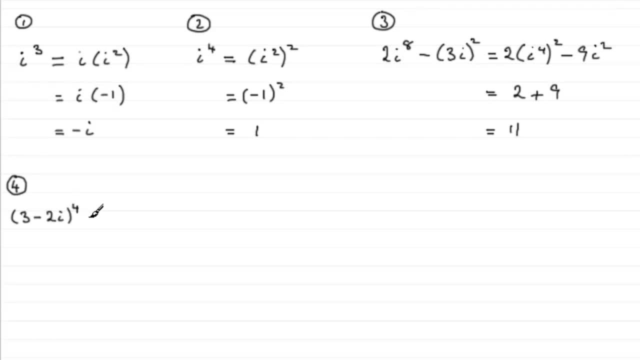 and I'm going to do it by the binomial expansion. and if you're unfamiliar with the binomial expansion, just go back on my website and look under the binomial expansion. but I'm assuming that you're familiar with this And I'm going to do it by the combinations method. 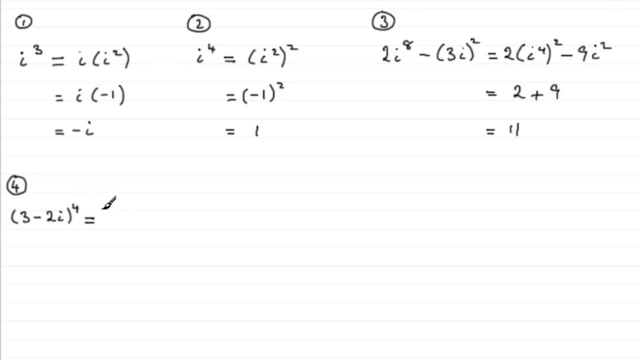 so what we have is first of all 4c0, and then we take the first term, in this case 3, and raise it to the power 4, and then we take the second term minus 2i, and that is to the power 0. Then for the 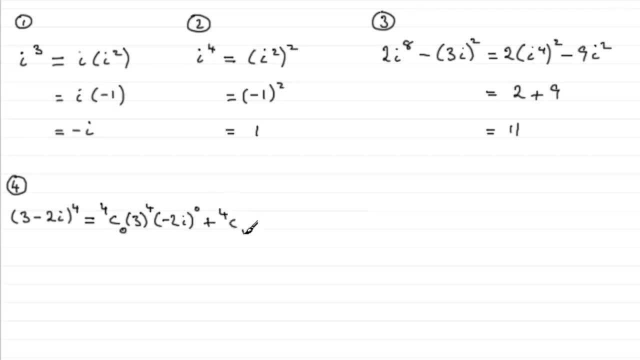 next term is 4c1.. Take the first term, reduce it by 1 in the power, so that's now to the power 3. take the second term minus 2i and increase that by 1 power, so that's now up to the power 1.. Next term: 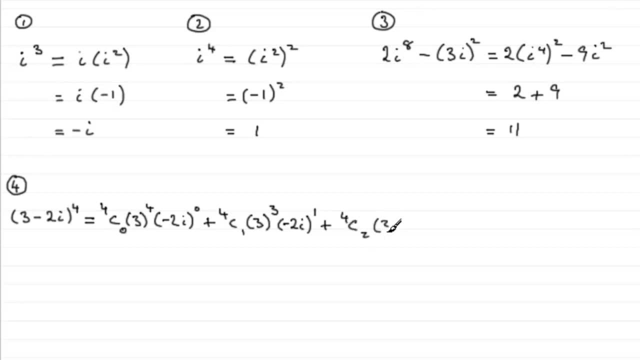 4c2.. Drop the power of the 3 by 1, so that's 3 squared. Increase the other one by 1, so that's now up to the power. 2. Start again for the next term. 3. Reduce the power 3 by 1, so that's 3 to the power 1. 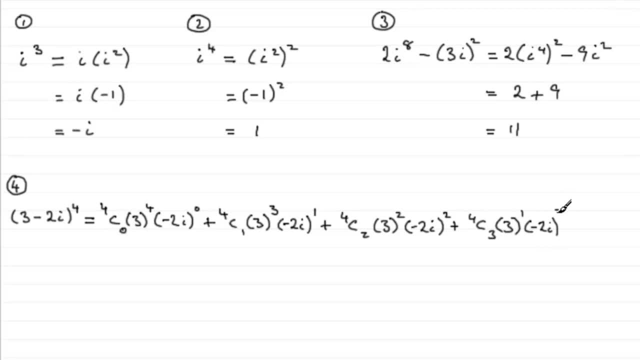 and then we've got minus 2i. Increase that now by 1, that's the power 3, and for the last term we've got 4c4: 3 to the power 0 and minus 2i to the power 4.. Now 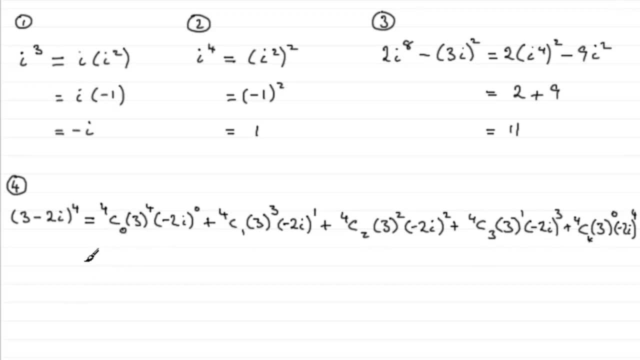 normally I'd go straight to the answer now, but what I'm going to do is put in another line where I just break down all the various parts, just so you can see what's happening. so 4c0 is 1, 3 to the power 4. well, that's going to be 81. 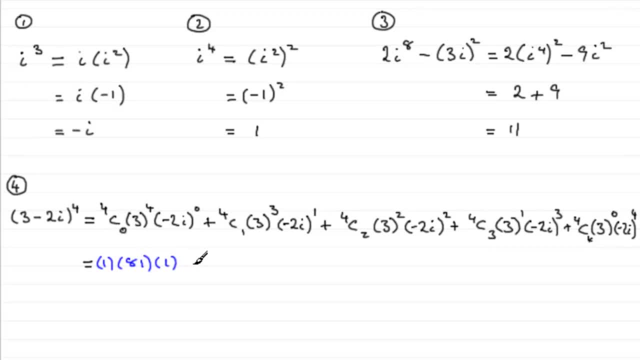 and anything to the power 0. well, that's going to be 1. when we come on to the next term, 4c1 is 4, 3 cubed is going to be 27. now, when we get this one, this is going to be minus 2i to the power 1. 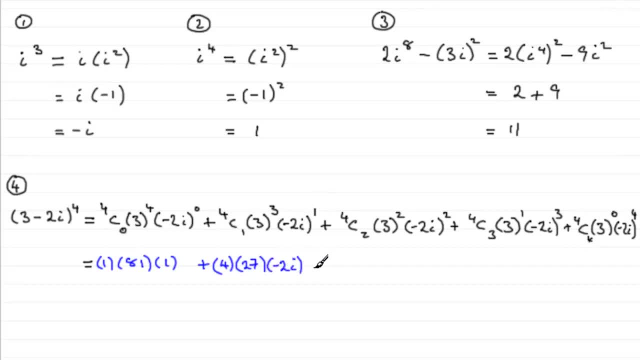 this is going to be minus 2i for the next term. we've got 4c2, which is six. three squared, we know is nine, and then when we get the minus 2i squared- well, minus 2, if you were to square- it is going to be four. 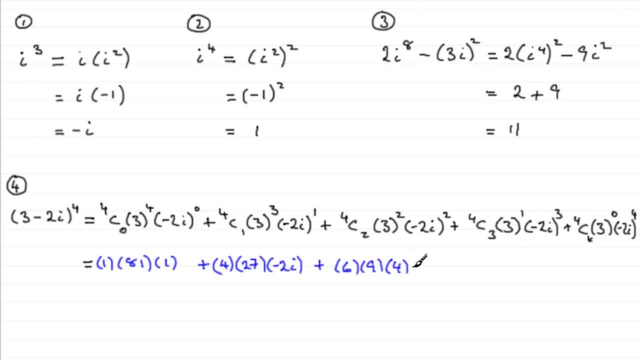 and then i: if you square, that is minus 1. now, when we have 4i to the power 4, have 4c3, that's 4. 3 to the power 1, well, that's 3. and now for minus 2i. all cubed, we've got the. 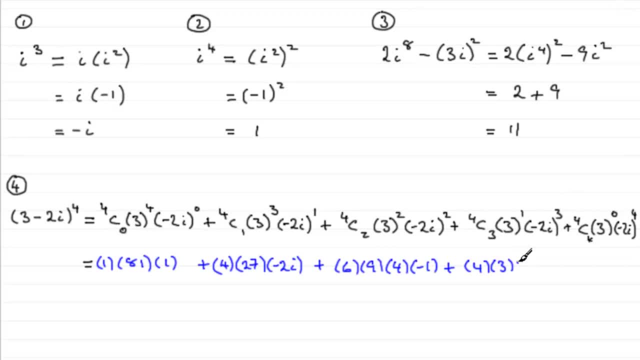 minus 2. if you were to cube, that is minus 8. and then you've got i, that is cubed. and if you cube i, we've seen that that result is minus i. so we've got minus i there, and then plus 4c4. well, that's 1. 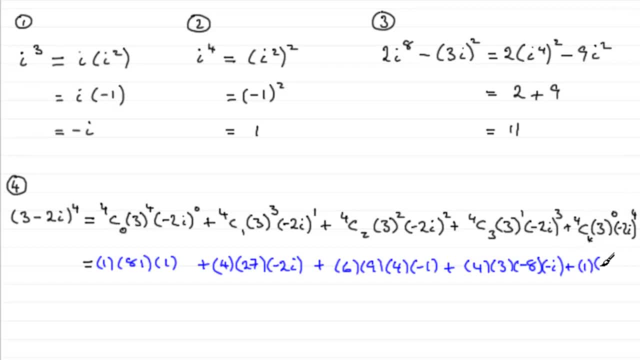 3 to the power 0, that's another 1. then you've got minus 2 to the power 4, which is going to be 16, and then you've got i to the power 4 and i to the power 4. we saw earlier was 1, so that's times 1. 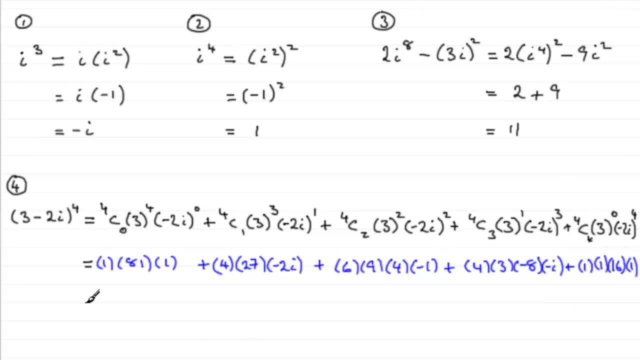 so if we were to clean up each of these terms now, what you end up with is 81, and then this one is minus 216i, and then for the next term you've got a minus and that is 216 for this term. here it's going to be plus. 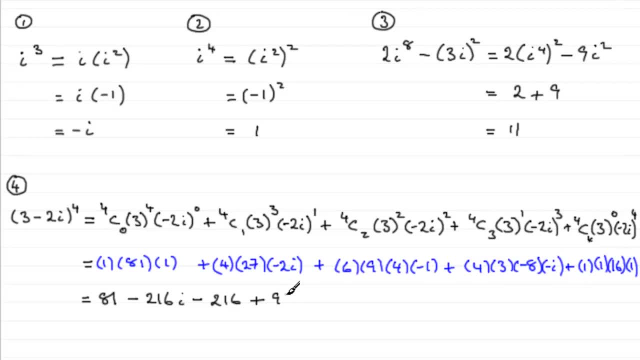 plus plus 96i, and then for the last term it'll be plus 16. so you're going to take care over those terms. very easy to get caught out on the signs. okay, just group together the real values 81 minus 216 plus 16. well, that gives us minus 119 and, for the imaginary parts, minus 269 plus. 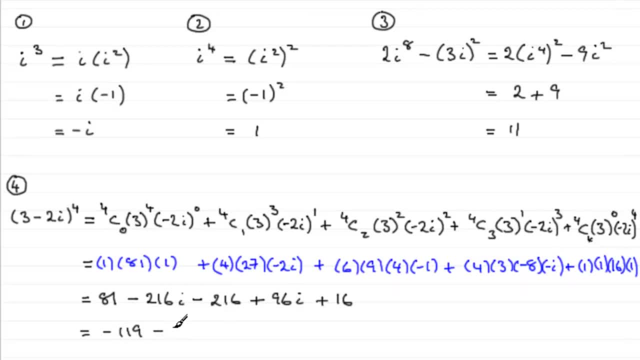 96, I like, gives us minus 120i. so hope you got that okay. but you could do it the long winded way by this, to say expanding 4 brackets. but I furniture the binomial expansion for something like this, okay. well, that brings us now to the end of this jury. son has given you some.